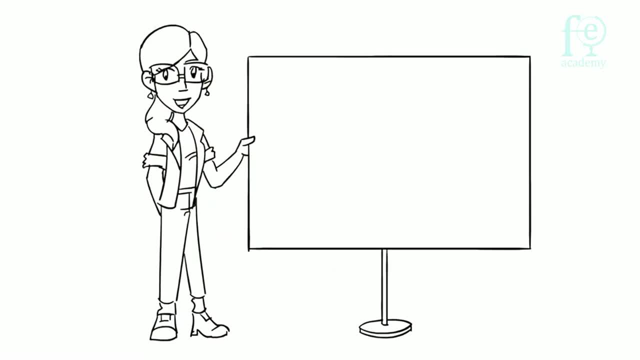 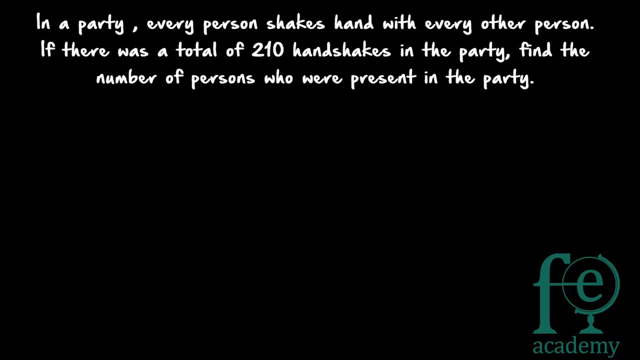 Hi friends, welcome to today's class. So today's question is: in a party, every person shakes hand with every other person. If there was a total of 210 handshakes in the party, find the number of persons who were present in the party. So this is a very common question asked for competitive exams. 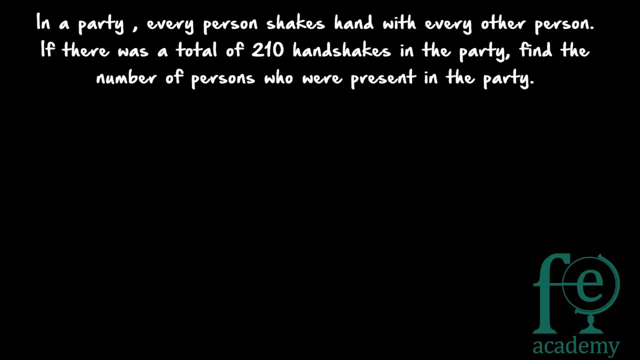 So there were seven people in a room, So every person shook hands with every other person. So how many handshakes were exchanged in that room? So likewise, many questions will come from this topic. So how to do this? So how many handshakes are there? Here, 210 handshakes are taking place. 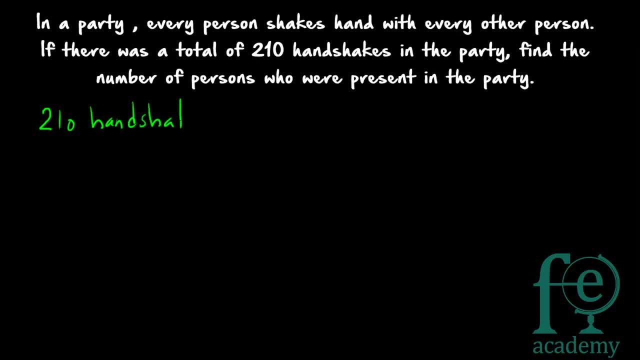 and you are asked to find out the number of persons in the room. So for this, suppose there are n persons For a handshake to take place, how many persons should be there? Two persons, Two people should come together and shake hands with each other. So it is a selection of two people. 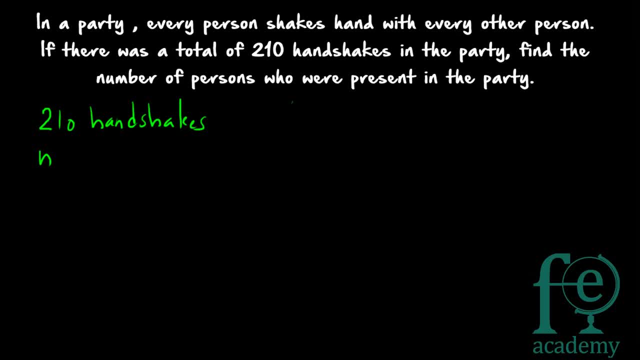 out of these n people. So here the order does not matter, Even if a is shaking hands with b or b is shaking hands with a, both are same only. So the order does not matter, It is just selection of two people out of these n people. So how many ways two people can be selected out of n people? 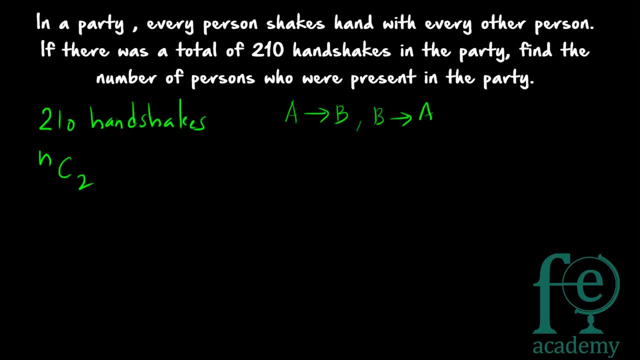 So out of n people, two people can be selected in n c 2 ways. So n c 2 is equal to 210.. So in every room with n people there will be n c 2 handshakes possible. Two people are coming together and shaking hands with each other. So how many ways two people can. 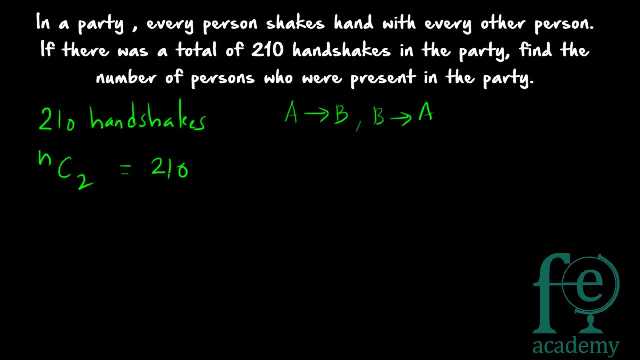 be selected out of these total n people. So it can be done in n c 2 ways Here. already it is given 210 handshakes are taking place in the party, So n c 2 is equal to 210.. Suppose the question is: 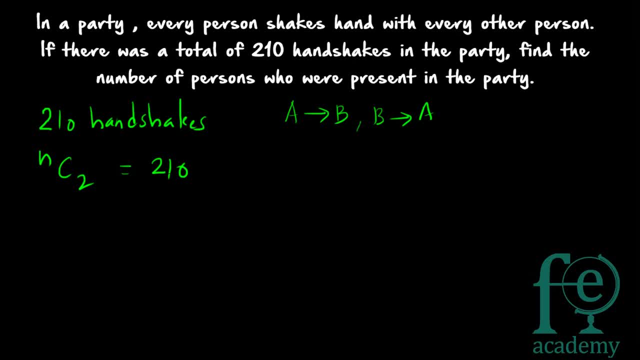 seven people are already in the room. So how many handshakes were exchanged? means it will be 7 c, 2.. So here it is. number of handshakes are given. This is a reverse question. You are asked to find out the number of people, So you 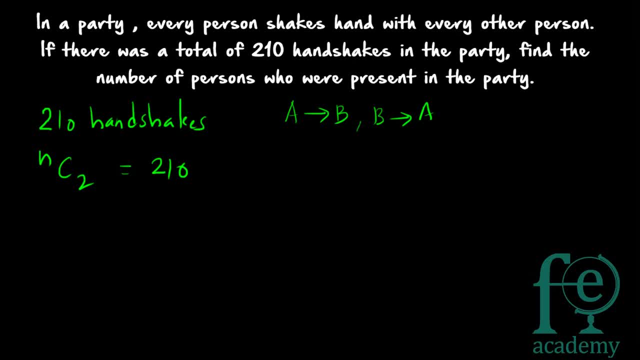 just remember: the number of handshakes possible if every person is shaking hand with every other person will be n c 2. It will be always equal to n c 2.. So if you are remembering this formula, you can easily find out the answer to these kind of questions. So n c 2 is equal to 210.. So 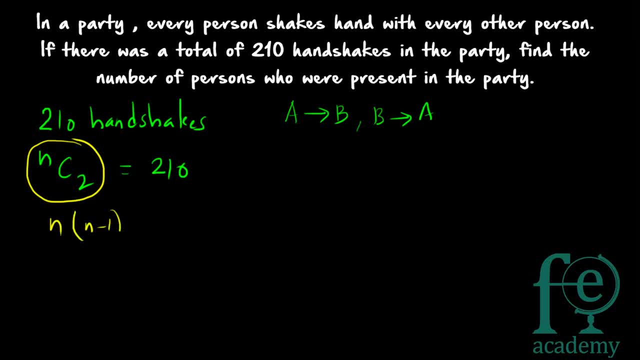 what is n c 2?? n c 2 means it is actually equal to n into n minus 1, divided by 1 into 2 is equal to 210, which will be giving you: n into n minus 1 is equal to 210, into 2 is equal to 420.. So n? square. 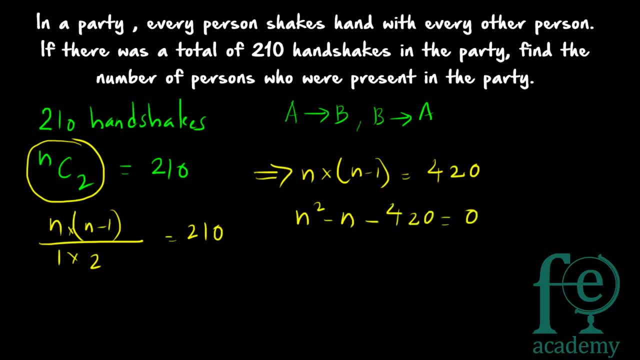 minus n minus 420 is equal to 0.. So what are the answers? You have to solve this equation: n square minus n minus 420 is equal to 0. So you will be getting n minus 21 into: n plus 20 is equal to 0 or n is equal to 21.. So there will be 21 people present in the party. 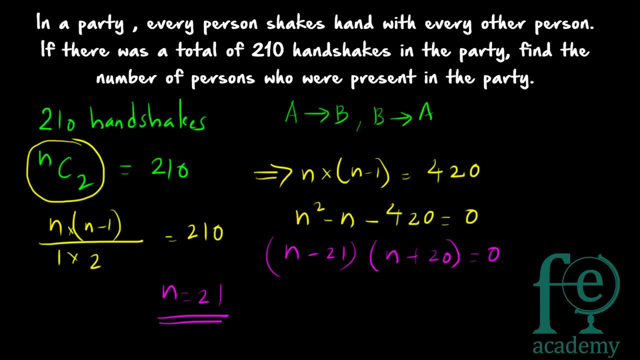 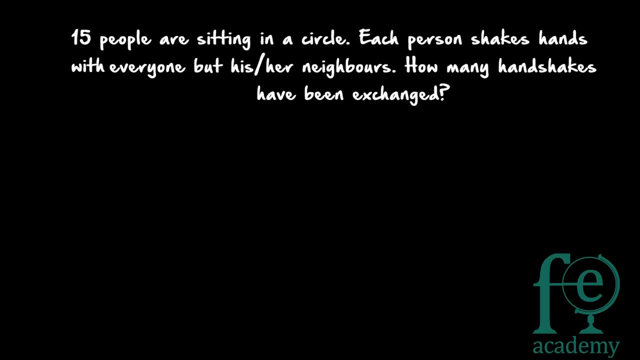 So a total of 210 handshakes will be exchanged. Second question: 15 people are sitting in a circle. each person shakes hands with everyone but his or her neighbors. How many handshakes have been exchanged? So 15 people are sitting in a circle. So 15 people are sitting in a circle and every 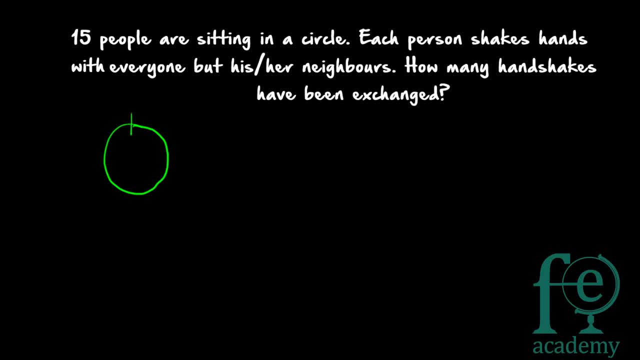 person shakes hands with his or her neighbors, So one person will not be shaking hands with his or her neighbor. So here suppose we are considering: a is sitting here, then b, c are sitting here, then d, e, f. likewise the 15 people are sitting. means this: a will not be shaking hands with b and c. 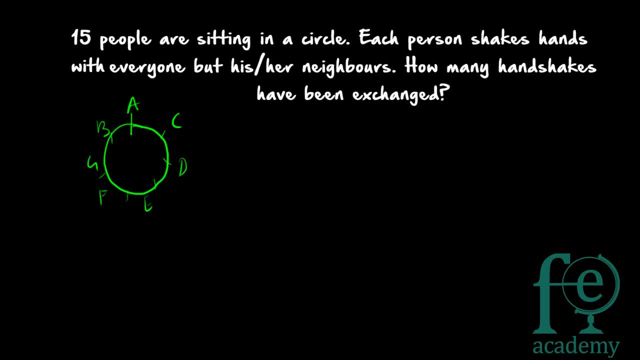 but with everyone else. a will be shaking hands, a will be shaking hands with d, a will be shaking hands with e, a will be shaking hands with f and so on, but a will not be shaking hands with b. So except his or her neighbors, A will be shaking hands with everyone else. 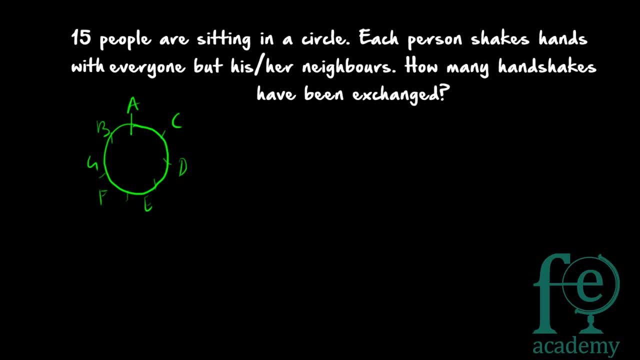 So how many handshakes have been exchanged? So first step is you have to find out totally how many handshakes are possible. So when there are N people, the number of handshakes possible will be equal to Nc2.. So here it will be equal to 15c2, which will be equal to 15 into 14, divided by 1 into 2. 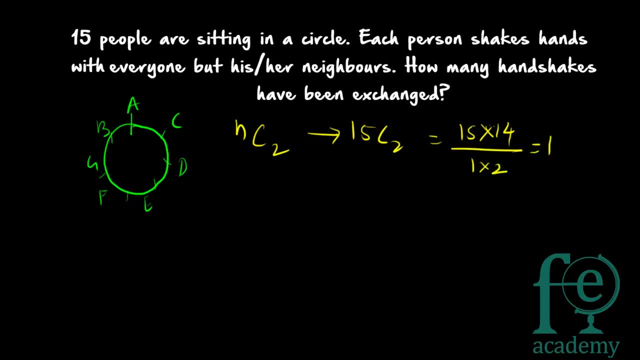 which gives you 15 into 7, is equal to 135.. So 135 handshakes are possible in total. and how many handshakes are not taking place? Each person is not shaking hands with two other persons. A is not shaking hands with B, as well as A is not shaking hands with C also. 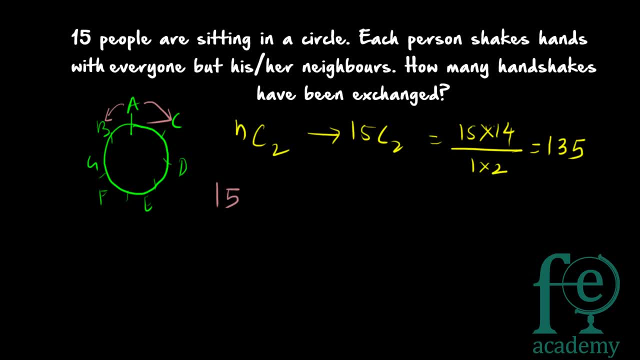 So 15 people will be shaking hands with. will not be shaking hands with how many persons? 15 into 2, but they are sitting in a circle, So A is not shaking hands with B and A is not shaking, So they are not shaking hands with C. 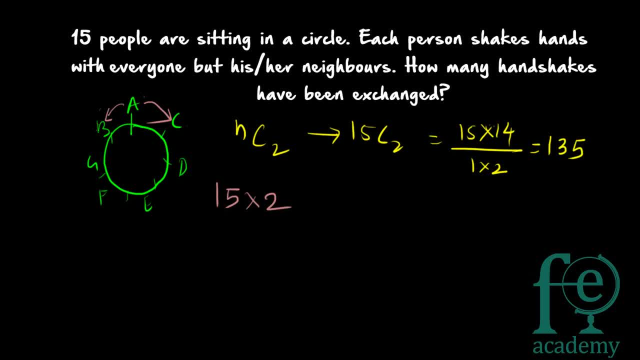 Similarly, B will not be shaking hands with A and B will not be shaking hands with G. So again, this A and B handshake is coming two times, So when we are considering the neighbors of A as well as we are considering the neighbors of B, 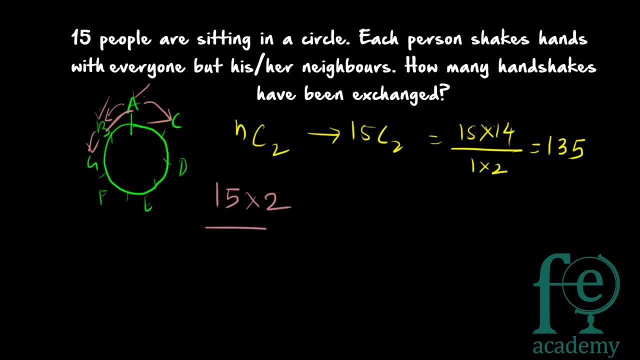 this single handshake is coming two times, So you have to divide by 2 in order to remove the duplicates. So 15 into 2, divided by 2, handshakes are not taking place, which means 15 handshakes are not taking place. 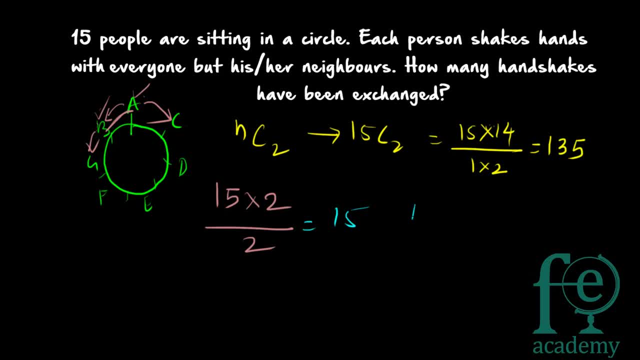 In total 15 handshakes are not taking place. So 135 minus 15, which gives you 120 handshakes will be taking place in total. So this also you can understand in a different way. There are 15 people and the 15 people. one person is shaking hands with 14 other people. 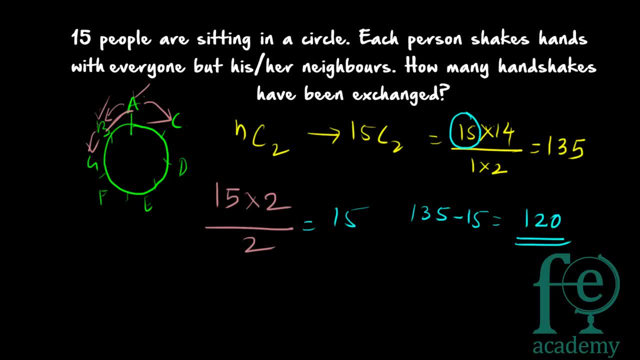 So 15 people will be shaking hands with 15 into 14.. So, in order to avoid duplicates, you have to divide by 2.. So that is how this formula came. Okay, One person will be shaking hands with 14 others, So 15 persons will be shaking hands with 15 into 14.. 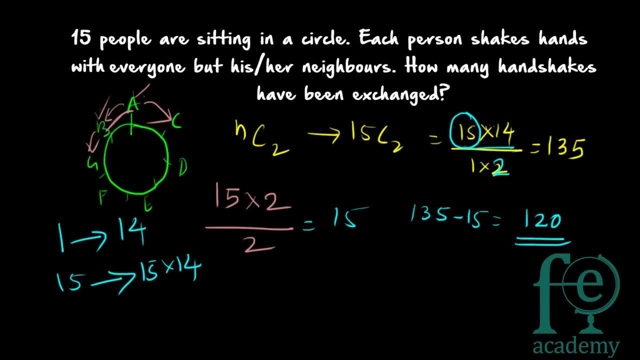 So 2 times one handshake will be taking place If you are forming the formula like this. So you have to divide by 2 in order to avoid the duplicates. So same concept only here also we are using: One person will not be shaking hands with 2 other persons. 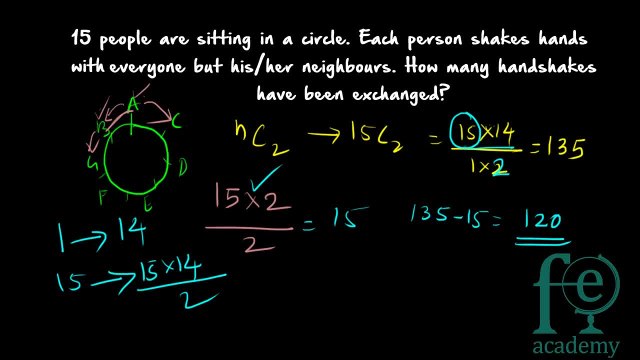 So 15 people will not be shaking hands with 15 into 2 persons. But in order to avoid duplicates, you have to divide by 2.. So it will be 15 into 2, divided by 2, which gives you 15.. 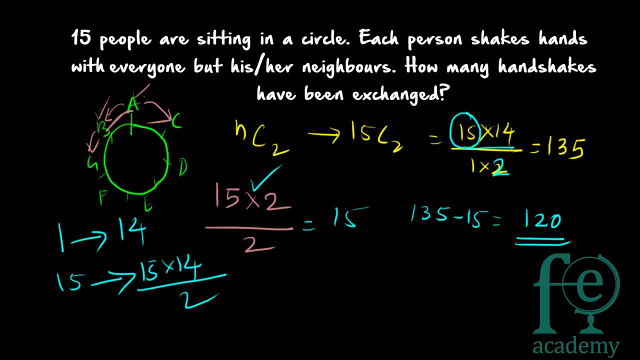 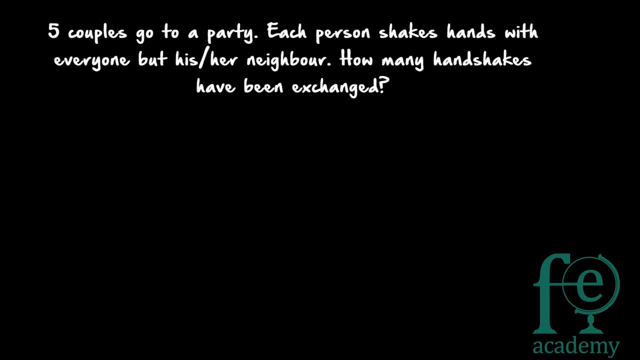 So in total 135 minus 15 handshakes which are not taking place. So there will be 120 handshakes taking place in that particular room. Now one more handshakes problem: 5 couples go to a party. Each person shakes hands with everyone but his or her spouse. 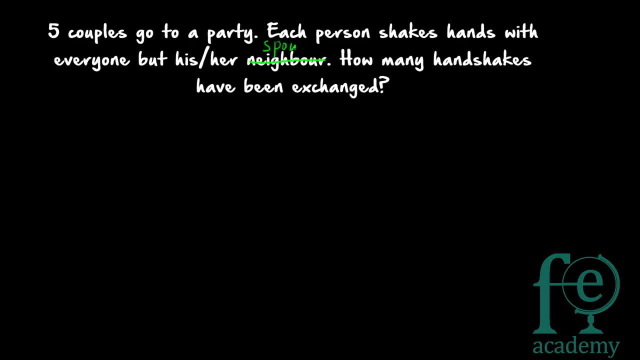 Okay, So sorry, it's not neighbor, it's spouse. How many handshakes have been exchanged? So 5 couples, or 10 people, are going to the party. So husband and wife, So 5. Couples, Okay, So 5 couples are going to the party. 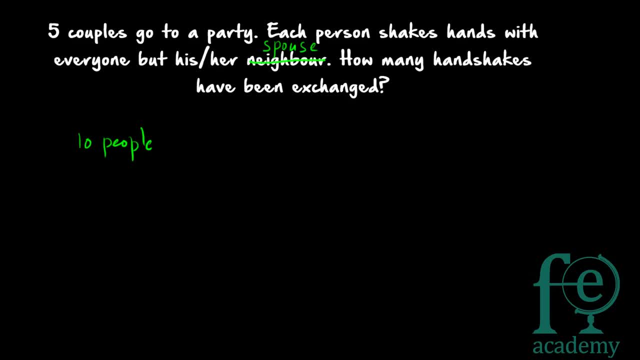 And each person will be shaking hands with everyone else in the room except his or her spouse. The husband will not be shaking hands with the wife And also the wife will not be shaking hands with the husband, But they will be shaking hands with everyone else. 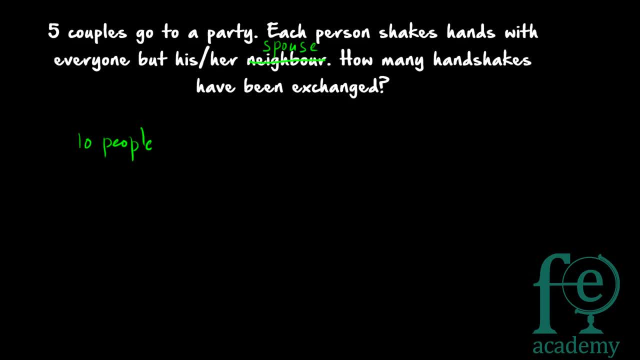 So how many handshakes have been exchanged? So here also you have to find out the total number of handshakes done. So there are 10 people. So you have to select 2 people each for the handshake to be done. So it can be done. 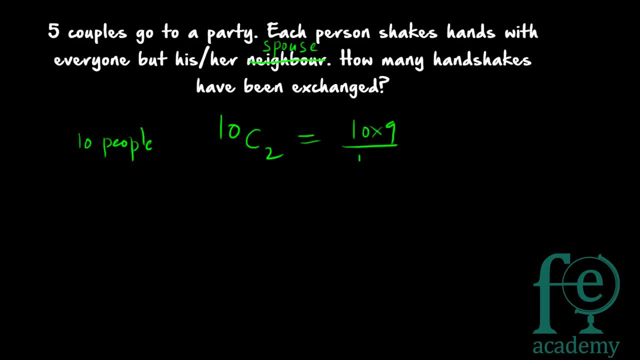 In 10 C2 ways, which will be giving you 10 into 9, divided by 1 into 2, which will be giving you 45. So 45 handshakes are possible in total. Then how many handshakes are not taking place? 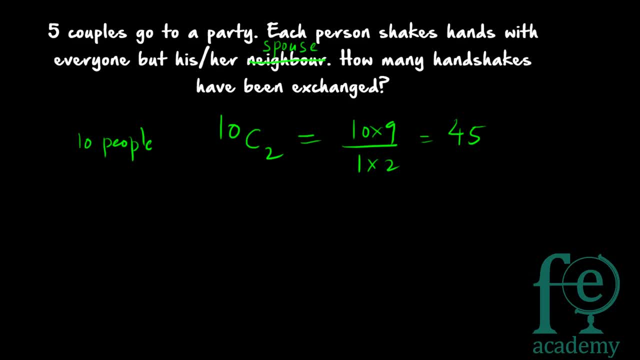 There are, 1 person will not be shaking hands with 1 another person, So 10 handshakes will not be possible, So you have to again divide by 2 in order to avoid duplication. 1 person will not be shaking hands with 1 another person. 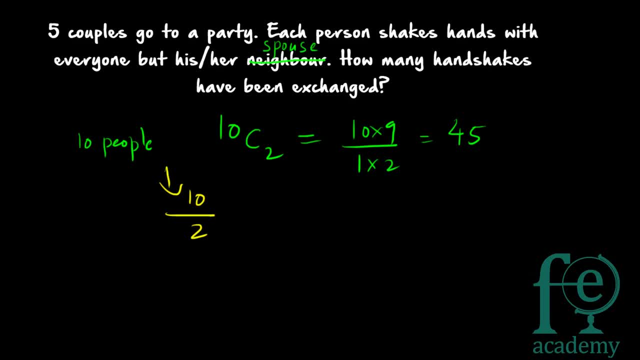 Husband will not be shaking hands with wife. Wife will not be shaking hands. Husband will not be shaking hands with husband, So 1 person will not be shaking hands with 1 another person. So 10 people will not be shaking hands with 10 people. 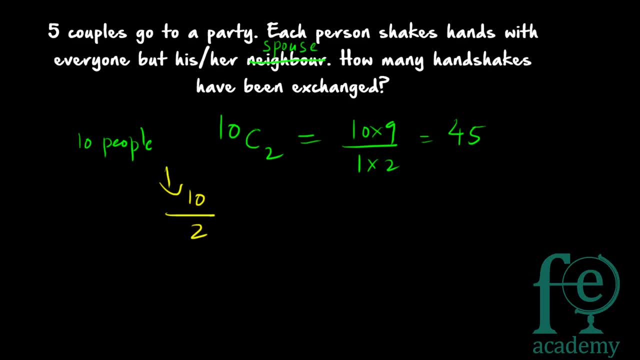 In order to avoid duplication, you have to divide by 2.. So 5 handshakes are not taking place. So in total, 45 minus 5 is equal to 40 handshakes have been exchanged in the party. Thank you for watching. 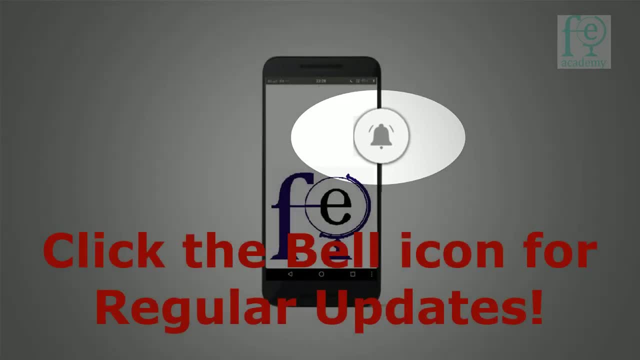 Please subscribe to my channel. See you in the next video.